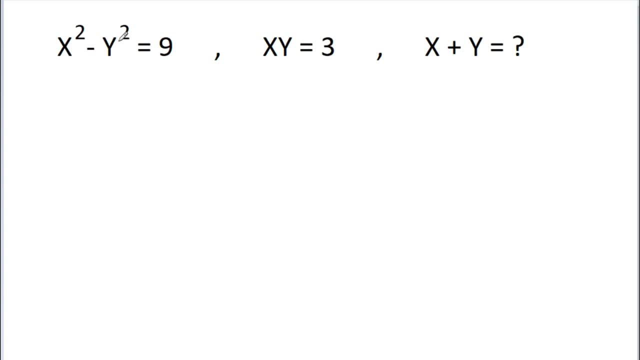 In this video we have given that x square minus y square is equal to 9 and x- y is equal to 3 and we have to find the value of x plus y. So here it is given that x square minus y square is equal to 9, and if we square it both side, then we get x square minus y square. 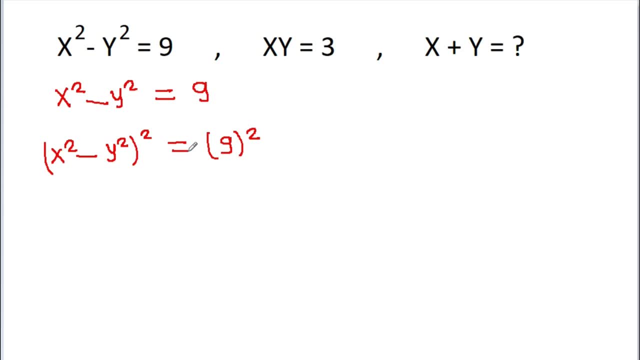 whole square is equal to 9 square and x square minus y square, whole square will be x to the power 4 plus y to the power, 4 minus 2 into x square into y square is equal to 9, square is 81. and now we get x to the power 4 plus y to the power, 4 minus 2 into here. x, y is equal to 3.. 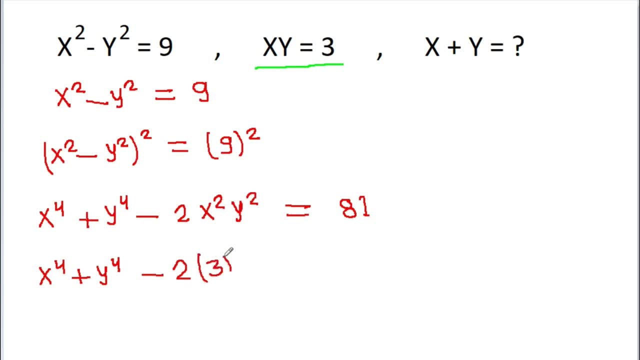 So x square, y square will be 3 square is equal to 81. and now we get x to the power 4 minus y to the power. 4 is equal to 81 plus 18, that will be 99.. Let's call this as equation 1. 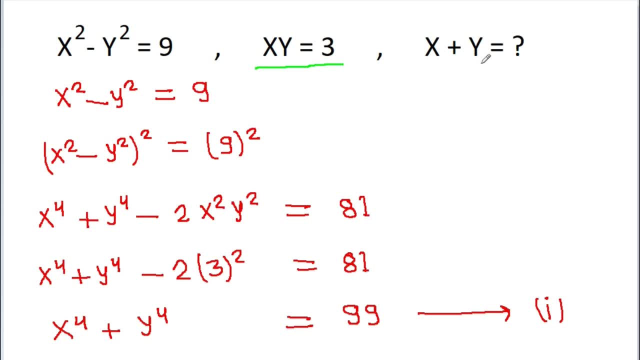 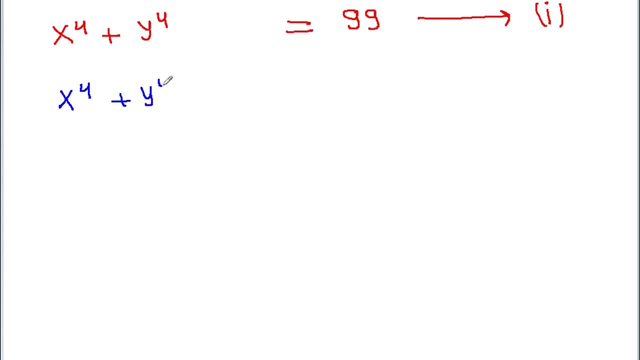 and now we have to find the value of x plus y. So x to the power 4 plus y to the power 4 is equal to x square plus y square, whole square minus 2 into x square, into y square, and we have x to the power 4 plus y to the power 4 is equal to 99.. 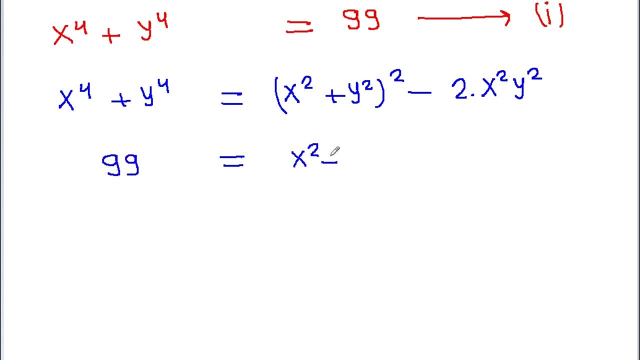 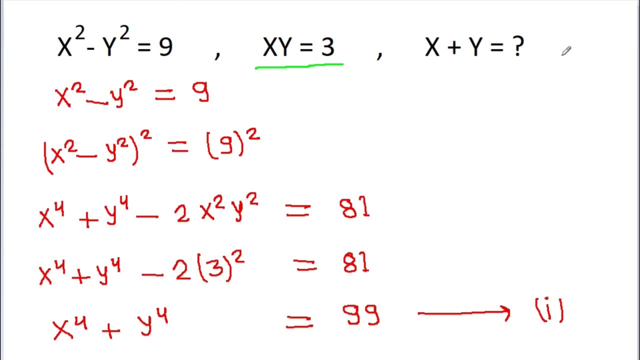 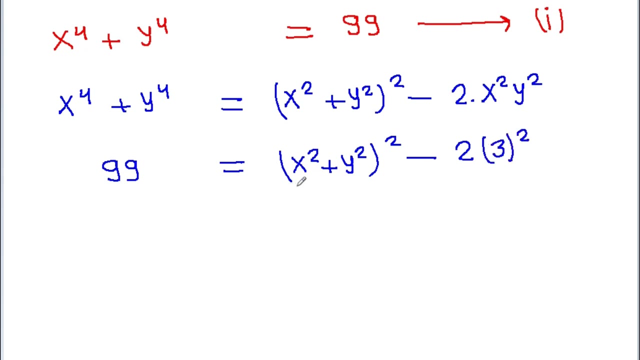 it is. 99 is equal to x square plus y square, whole square minus 2 times The value of x. y is 3.. So x squared, y squared will be 3 squared favor and from here we can get x square plus y square. whole square is equal to 99 plus 18. that will 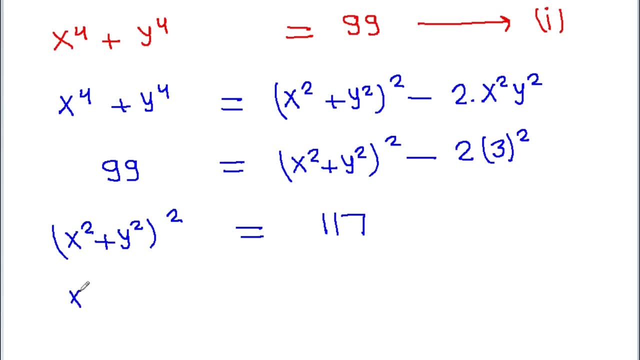 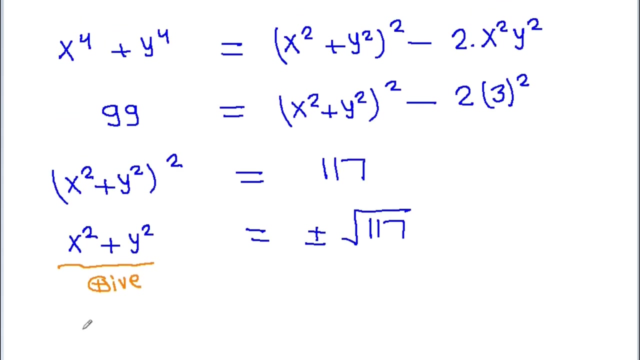 be 117, or x square plus y square will be plus minus root under 117, and here x square plus y square will be positive. so x square plus y square cannot be equal to negative root 117. so here we get: x square plus y square is equal to positive root 117. let's call this as equation 2.